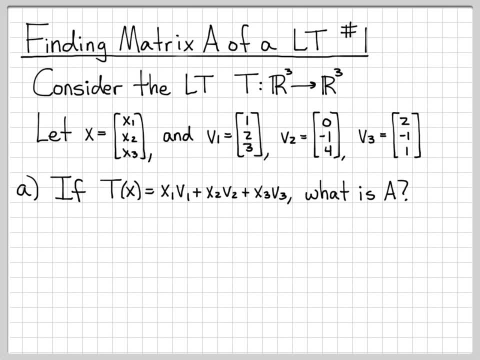 how this linear transformation operates. what is A? How do we represent this linear transformation? as a matrix operation on a vector x? So we would like to be able to write our linear transformation like this: We would like to be able to write: T of x is equal to some matrix. 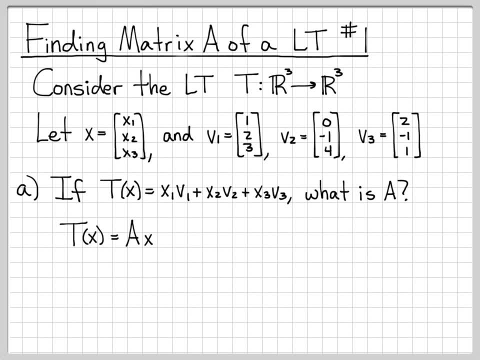 A, which we don't know, times the vector x. That's what we would like to do. We would like to find out what this matrix A is. Well, look at this: If A happens to be the matrix comprised of the vectors v1,, v2, and v3 as the columns, so v1 is the first column, v2. 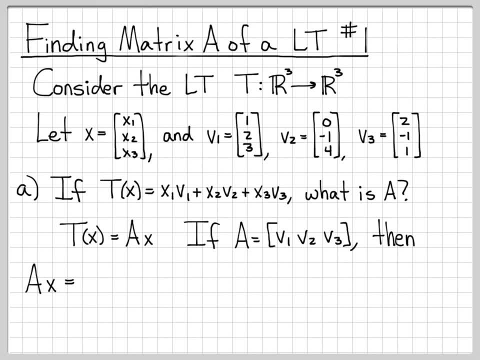 is the second column and v3 is the third column, then we can go ahead and compute. Let's just compute what this would be. So A x would be v1,, v2,, v3 times the vector x. Well, we know how to do matrix-vector multiplication. Each entry of the vector x is x1,, x2, x3 times. 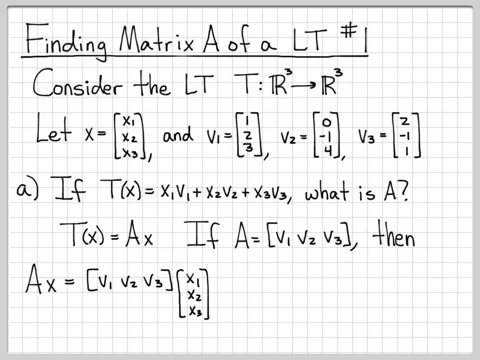 multiplies each column vector of the matrix A. So this is equal to v1- x1, the first element of x times the first column of A, plus x2 times the second column of A, plus x3 times the second column or the third column of A. So I wrote this a little different. it probably would have been. 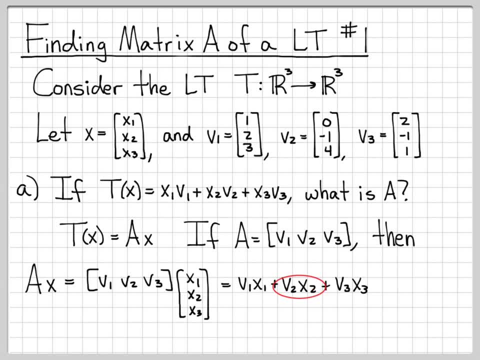 more appropriate to write it as x1- v1, and x2- v2, and x3- v3, because that's how we define scalar multiplication. But it's clear here what we're doing. this is just the vector v1, with every. 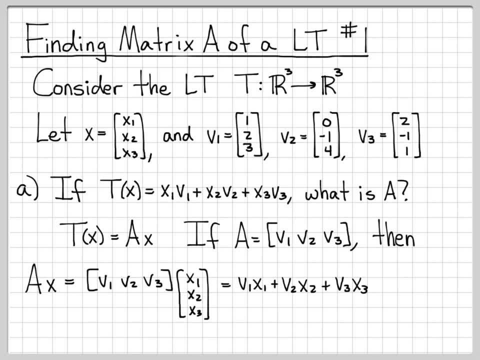 entry scaled by x1, etc. So this is equal to x1 v1 plus x2 v2 plus x3 v3.. This is exactly what we wanted to achieve. we wanted to have x1 v1,, x2 v2, and x3 v3.. So I kind of took a stack. 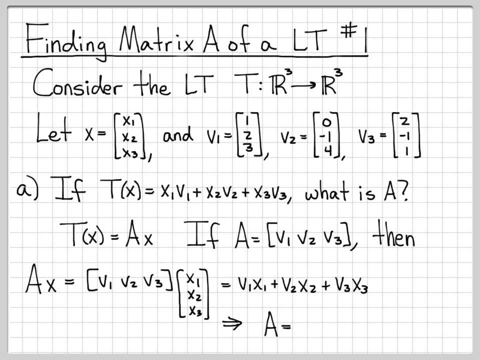 what I thought A1 might be, and that turns out. this matrix right here is exactly what it needs to be. We constructed the matrix A and it turns out it yielded the exact transformation that we wanted. So A should be the matrix whose first column is v1,, whose second column is v2, and whose 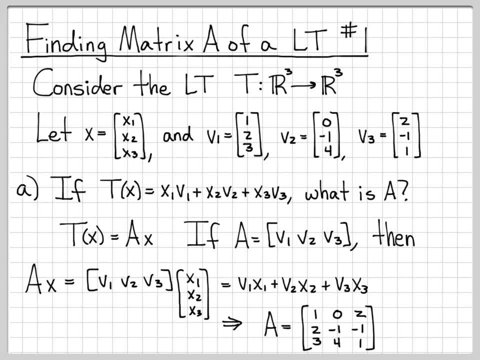 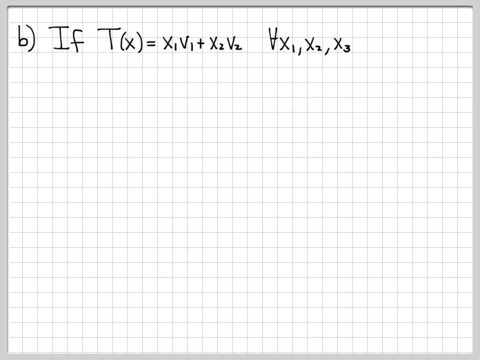 third column is v3.. This is the matrix representation for the linear transformation defined by this operation. right here Let's do another little example. What if t of x? the linear transformation was defined like this: So this is a little bit different. Now I'm saying that the linear transformation takes an input. 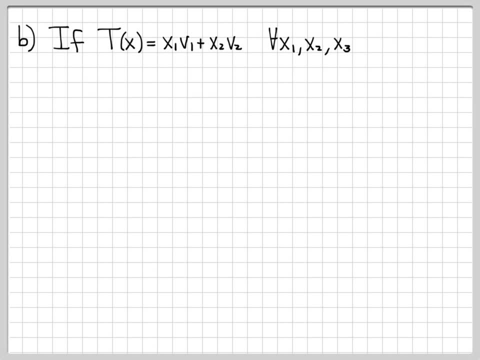 vector x and it returns the x1 times v1 plus x2 times v2.. This is a little bit different. There is no x3 or v3 here, it's only x1, v1 and x2 v2.. So in this case, what would A be? Well? 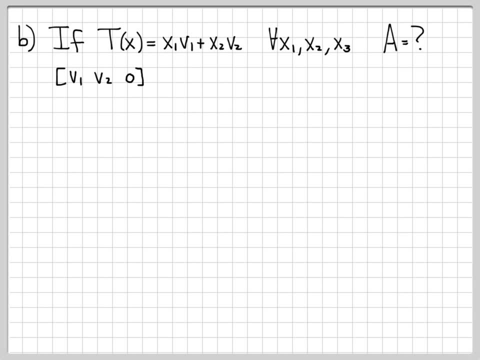 it's pretty easy to guess what it should be. Let's take a stab at it and say that A is the matrix whose first column is v1,, whose second column is v2, and whose third column is the all-zero vector. So this is a vector of zeros, the column vector, and for this particular 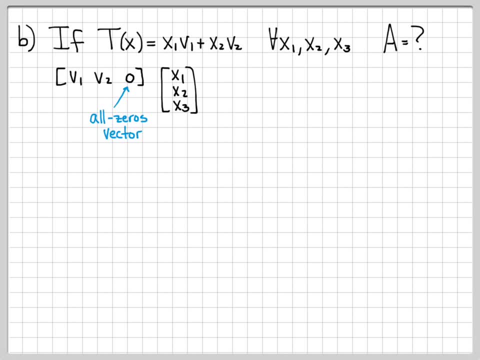 example, it has three zeros in it. If I multiply this by my vector x, what do I get? I get x1, v1 plus x2, v2 plus x3 times the all-zero vector, which gives us an all-zero vector which, when 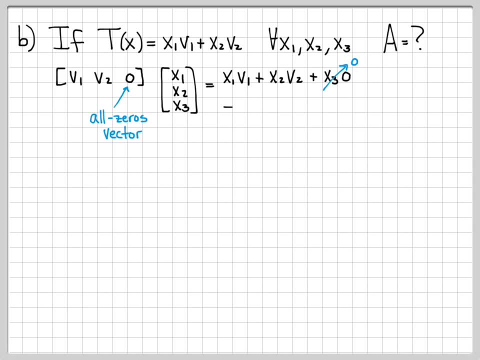 added to these other vectors doesn't change anything. it just goes to zero. So I end up with just x1- v1 plus x2 v2.. So I've kind of guessed what I think A should be, and we have verified that it does give us the transformation of x, as stated in the problem. 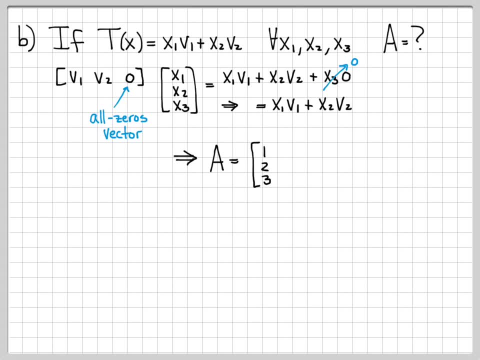 right here. So for this example, A would be 1,, 2,, 3,, 0, negative 1, 4,, because that's what a v2 is, and that its third column would be the all-zero vector. So this was a little simple example. 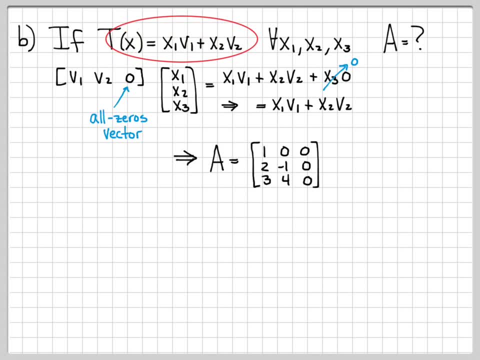 of when you're given kind of the equation for how the linear transformation works, how you go about kind of guessing at the form of A. Often A is comprised of the vectors that you're given. You just kind of have to multiply it out and verify that that is the case.